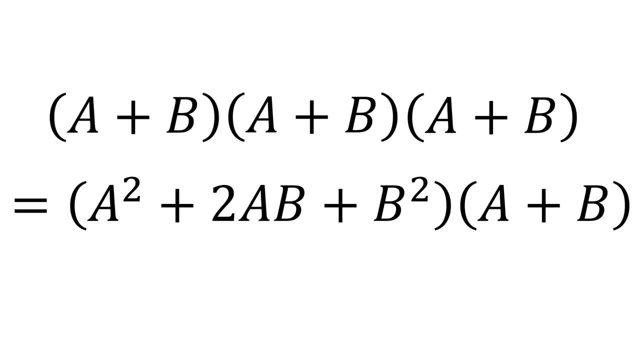 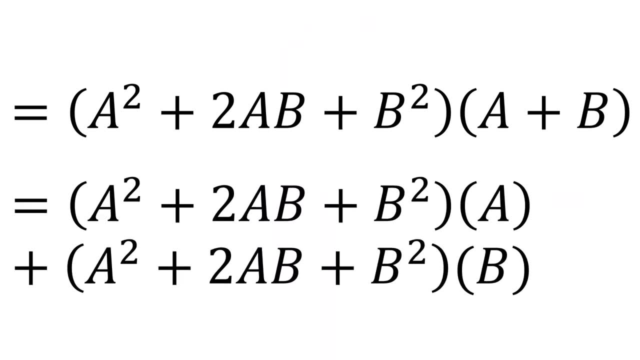 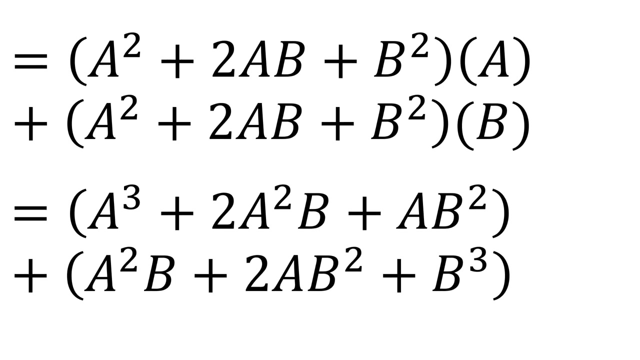 times a plus b. By distributive property, this is equal to a squared plus 2ab plus b squared times a plus a squared plus 2ab plus b squared times b. Using distributive property, once again, this equals a cubed plus 2ab squared b plus ab squared plus a squared b. 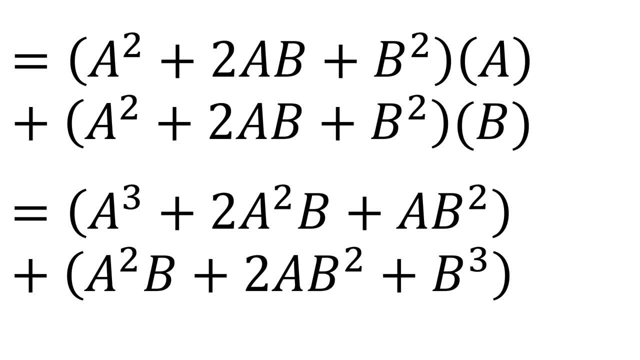 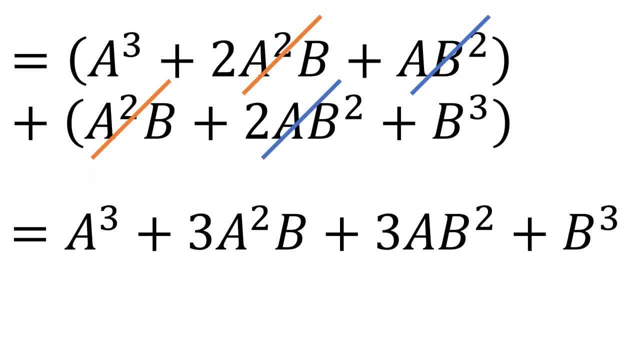 plus 2ab squared b plus 2ab squared b. Combining like terms, this equals a squared plus 3a squared b plus 3ab squared plus b. cubed times: a plus 3ab squared plus 3ab squared b plus 3ab squared plus 3ab squared, So therefor: 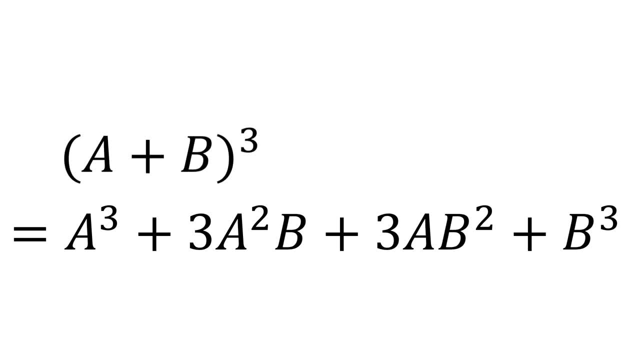 the cube of a plus b is equal to a cubed plus 3 a squared b plus 3ab squared plus b cubed. Now, using this formula, we can quickly find the cube of this cube sum of two terms without using the FOIL method or the distributive property in general. 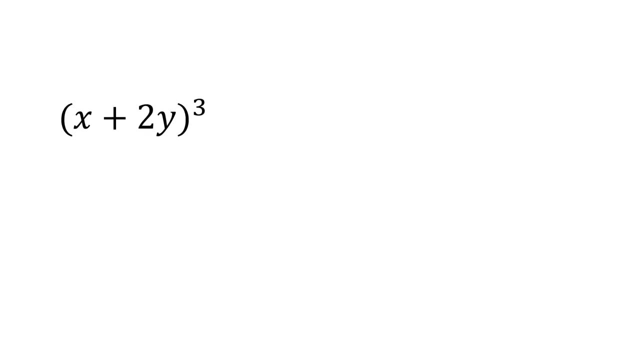 For example, let's say we have x plus 2y cubed. In this case we have a as x and b as 2y. Now, instead of using the FOIL method, just take the cube of x plus 3 times the product. 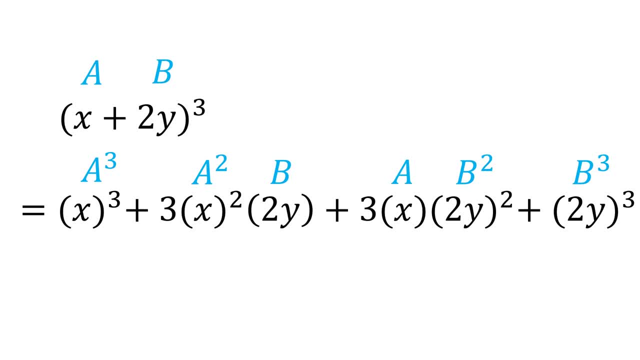 of square of x and 2y plus 3 times the product of x and square of 2y plus the cube of 2y, which is equal to x cubed plus 6x squared y plus 6xy squared plus 8y cubed. So therefore, 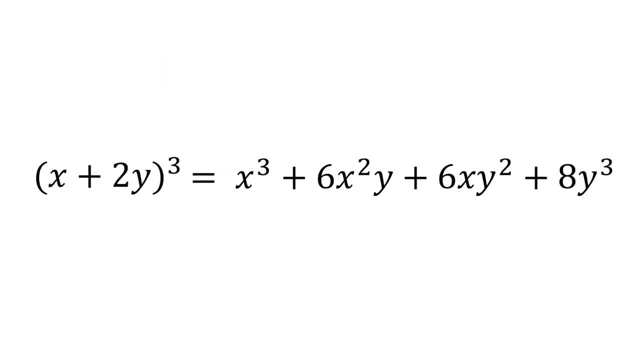 x plus 2y cubed is equal to x cubed plus 6x squared y plus 6xy squared plus 6xy squared plus 8y cubed. Now let's say we have 3x plus 1 cubed. In this case we have a as 3x and b as 1.. 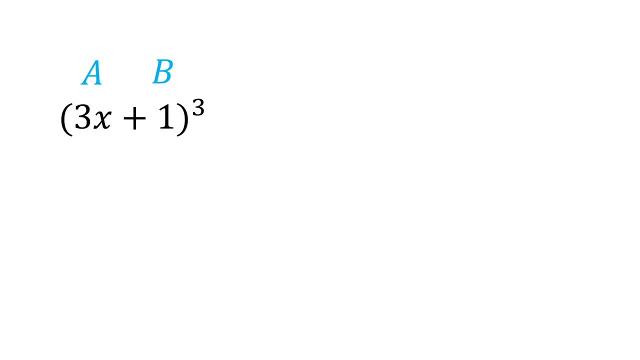 Now, instead of using the FOIL method, just take the cube of 3x plus 3 times the product of square of 3x and 1, plus 3 times the product of 3x and square of 1, plus the cube of 1,, which is equal. 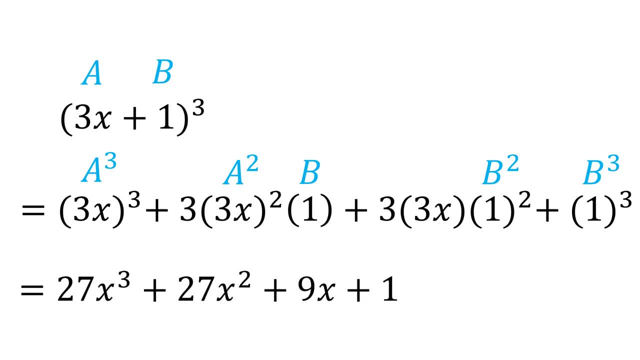 to 27x cubed plus 27x squared plus 9x plus 1.. So therefore, 3x plus 1 cubed is equal to 27x cubed plus 27x squared plus 9x plus 1.. 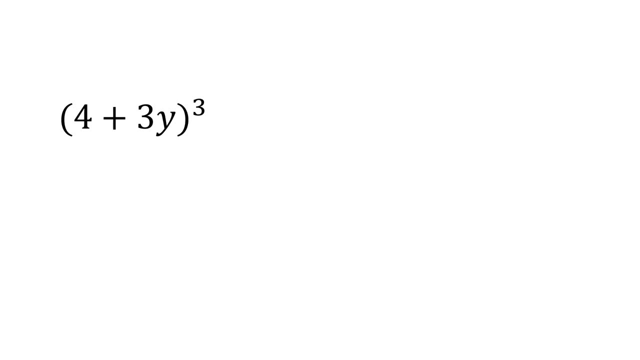 If we have 4x plus 3y cubed, then we have a as 4 and b as 3y. Now, instead of using the FOIL method, just take the cube of 4 plus 3 times the product of square of 4 and 3y plus 3 times the product. 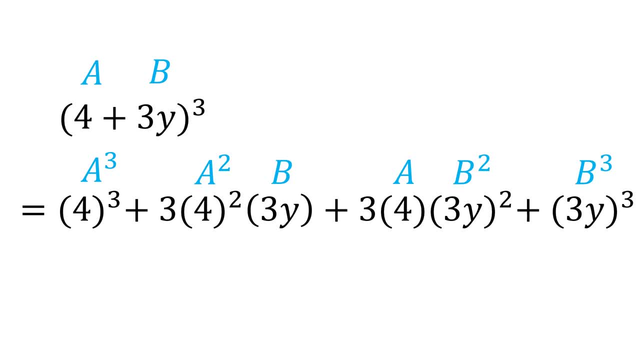 of 4 and square of 3y plus the cube of 3y, which is equal to 64 plus 144y plus 108y squared plus 27y cubed. So therefore, 4 plus 3y cubed is equal to 64 plus 144y plus 108y squared. 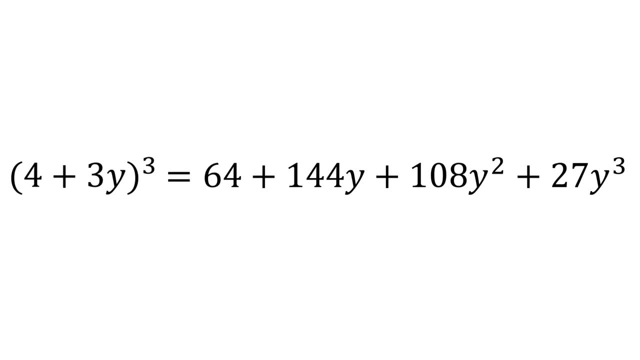 plus 27y cubed. Now I hope you get the idea on how to get the cube of the sum of two terms by recognizing it as a special product. Thanks for watching. 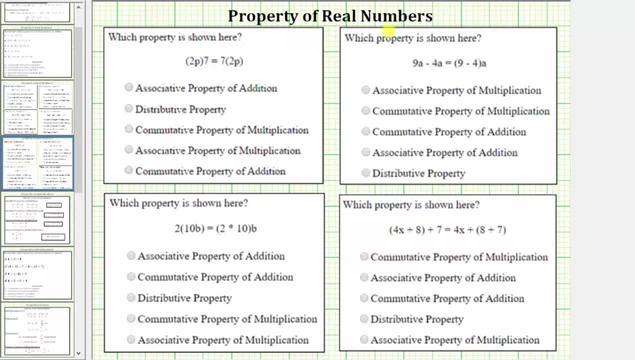 Welcome to four examples of determining which property of real numbers is shown. In the first example we have the quantity 2p times 7 equals 7 times the quantity 2p. Notice: on both sides of the equation we have a product, but on the left side we have the 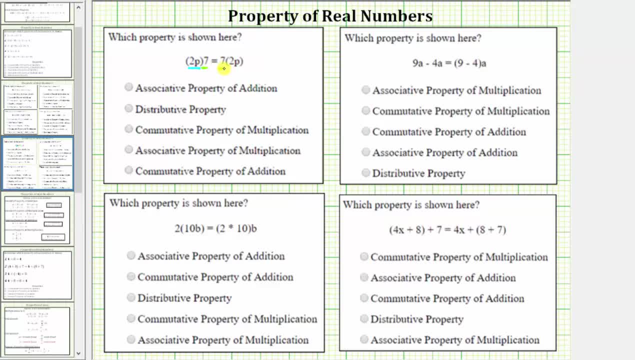 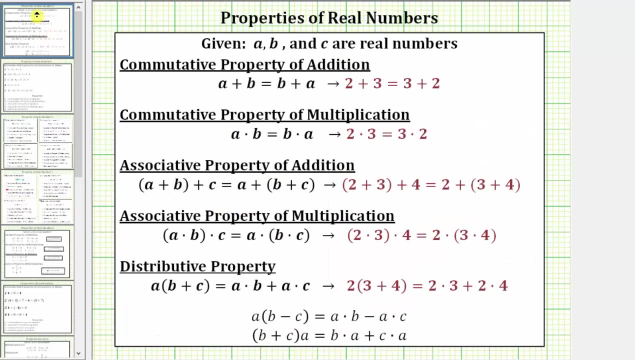 quantity 2p times 7, on the right side we have 7 times the quantity 2p. The order of the multiplication has changed, which is the commutative property of multiplication. This is normally expressed more formally as a times b equals b times a.